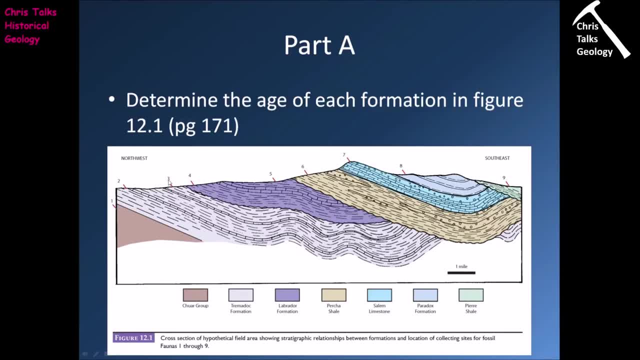 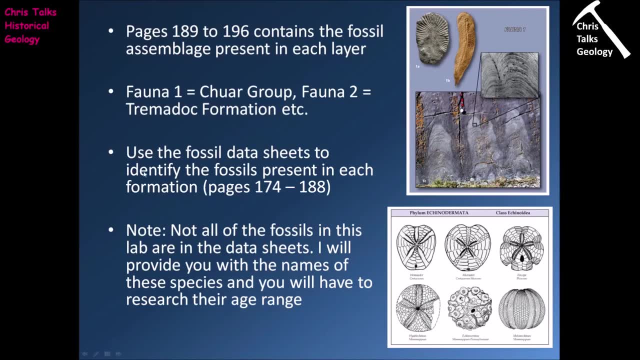 correspond to location 2, fauna 3 will correspond to location 3, etc. So what you're going to do is you're going to use the fossil data sheets to identify the fossils, and by doing so, you are then going to be able to date each layer of rock. Now the fossil sheets are are available on pages. 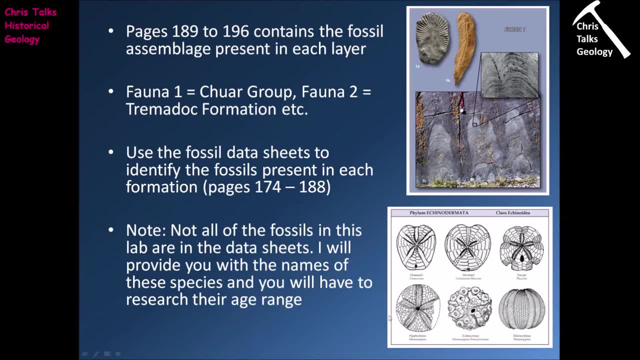 174 to pages 188, and you've already looked at them in the past. They're the sheets that look like this. Now you need to note that not all of the fossils in this lab are on the fossil data sheets, So there are about six or seven fossils which are not in the textbook. So at the end of this, 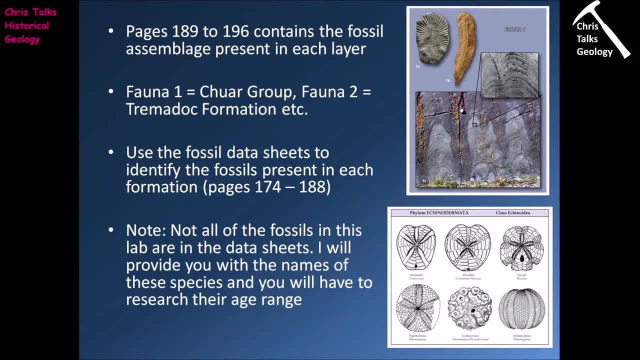 presentation. there's actually a list of these fossils and what you're going to have to do is you're going to have to research their age. So I'll give you the names of them, but you're going to have to work out. you know what periods of geologic time you're going to have to work out. 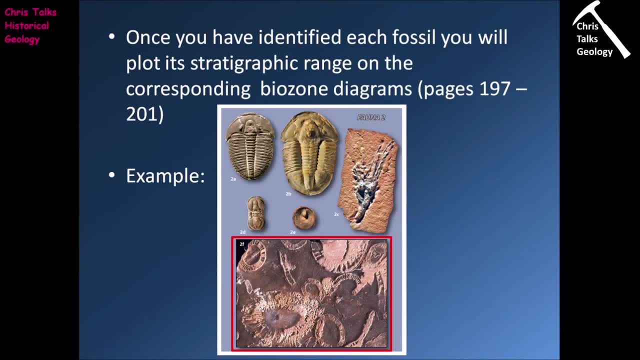 time they lived in. So once you've identified each fossil, you're going to plot its by, essentially its stratigraphic range on a biozone diagram and you're going to find these diagrams on pages 197 through to pages 201.. So this is going to be an example for fauna number two. So we're going to 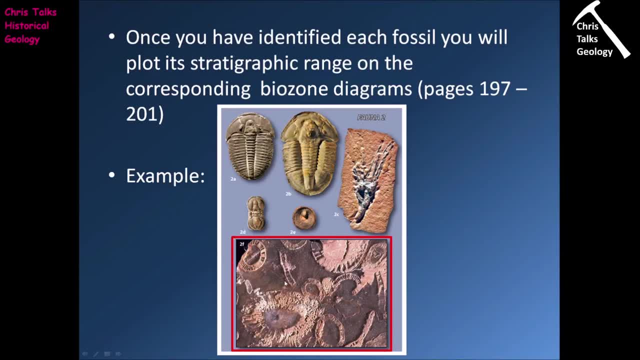 focus on this fossil here: 2f. So you can see you have these circular features and you can see it has this essentially this appearance of a 2f. So you can see you have these circular features and you can see it has this essentially this appearance. 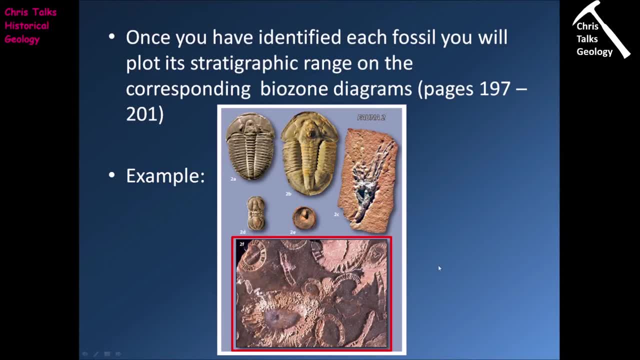 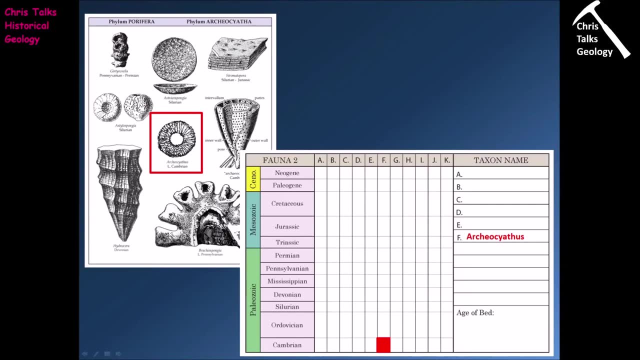 like it's split into lots and lots of smaller segments. So if we go to the fossil data sheets and we have a look through up, there's a circle right there and we can see once again it's split into these little segments. So now we've identified our organism, so obviously we have the species name. 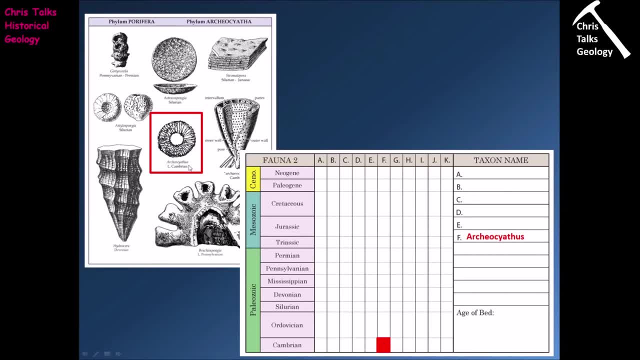 in italics, and we have the age- essentially the age range for that organism, below the species name. So what we're going to do with that information is we're going to come over here and we're going to put it onto a biozone diagram. Now, to begin with, make sure that you have the correct 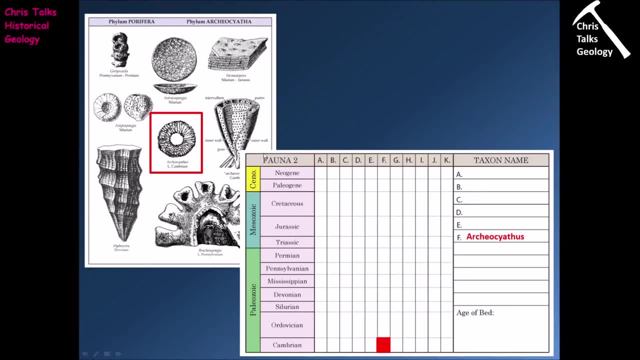 location. So we know that this, this biozone diagram, is for fauna number two and obviously you can see that's what we're looking at here: fauna number two. So we have the correct diagram for the correct fossil assemblage. So what you're going to do is you're going to write the name of 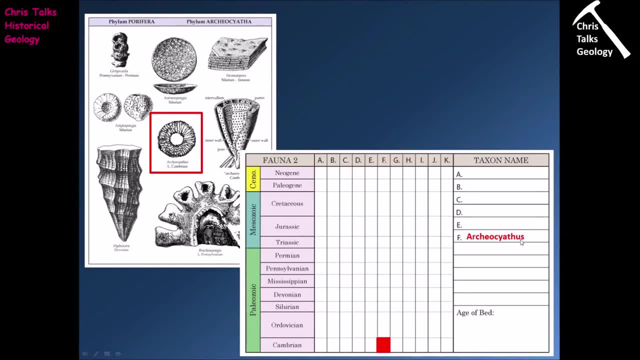 your fossil here. so obviously we were looking at fossil 2f, so the name's going to be written in there. it just makes it a little bit easier for me to mark. and then you're going to mark the age range for that organism on the diagram. so in the case of this organism it's essentially its age range. 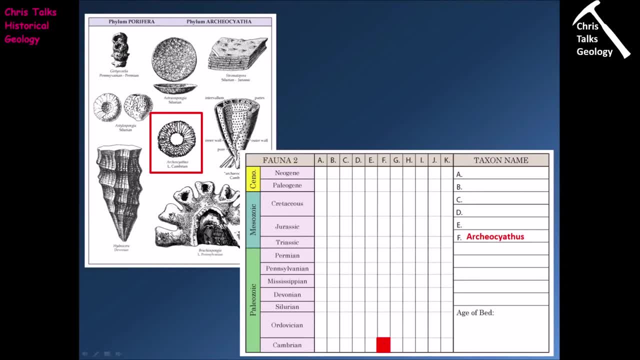 was lower cambrian only now. we don't really care about it when it says upper cambrian, lower cambrian or middle cambrian on the diagram here. so just simply fill in the entire cambrian box there and obviously you'll do this for each of the different species within that particular fossil. 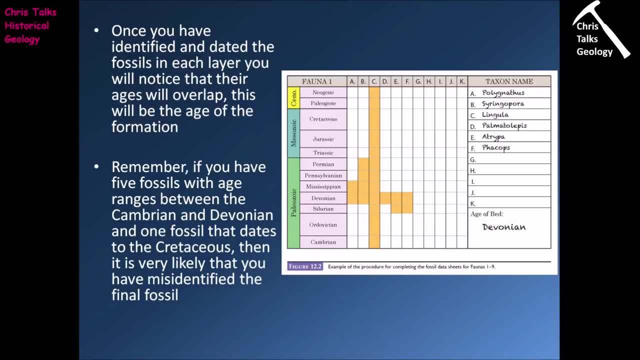 assemblage. so once you've identified and dated the fossils in each of the layers, what you're going to notice is that the age ranges for the fossils will overlap, and this is going to be the age of your formation. so this is a example taken from the textbook and you can see we have, uh, we've. 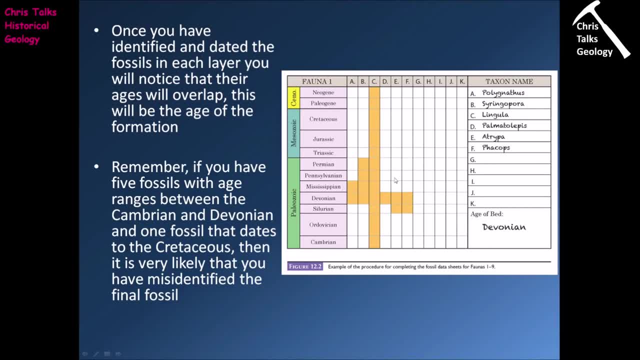 got one, two, three, four, five, six. we have six different fossils, and the age ranges are marked out here in orange, and what you're going to notice is that all of the fossils essentially overlap here in the devonian, and so this is going to be the age of your layer, because, remember your layer. 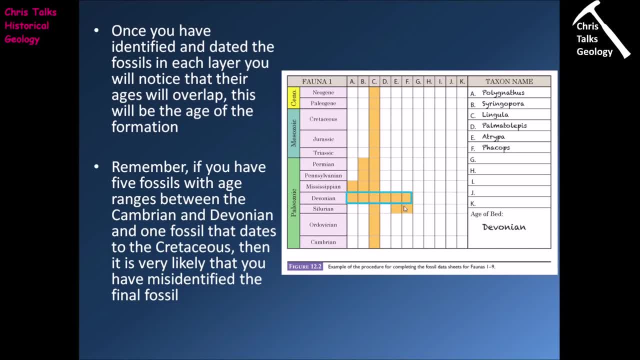 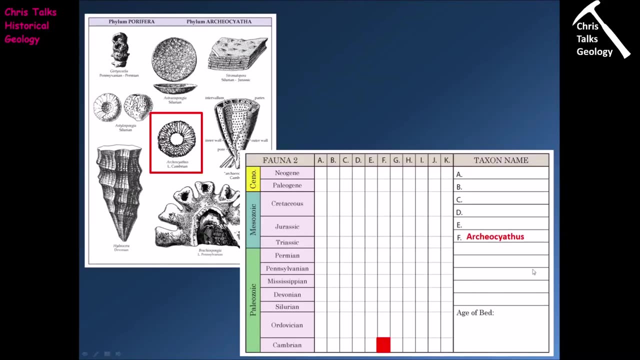 can only date the devonian, because the devonian is the only time when all of these fossils could have coexisted together. now, obviously, you're also going to write the age of your bed here in the diagram. so if we just go back to the previous slide, you'll notice that this area is 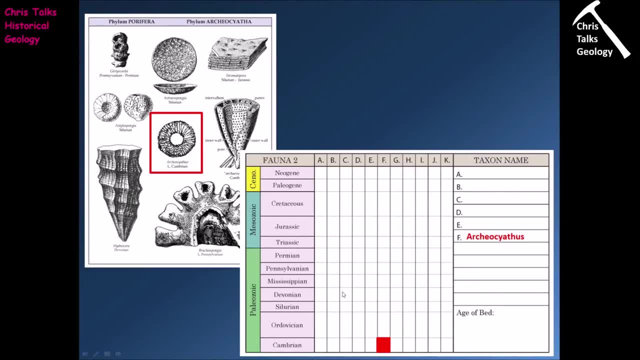 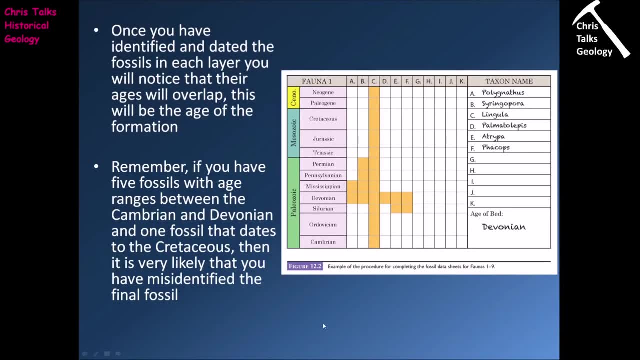 blank. so once you've identified all of your fossils, you've drawn their range zones on the diagram here. you can then work out what the age for that location is. now you need to remember that if you have five fossils with an age range between the cambrian and devonian and you have one fossil, 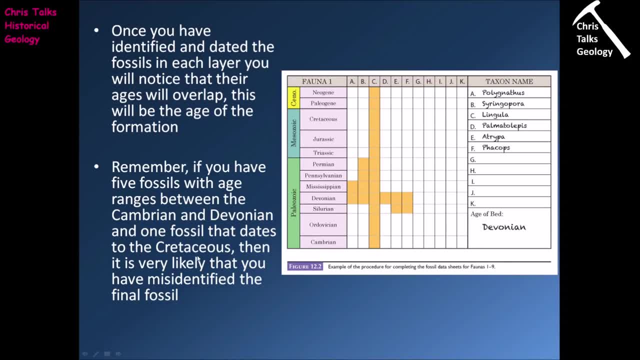 that you identify from that location and that fossil dates to the cretaceous, well then it's very likely that you've misidentified the final fossil. so just try and be smart. so if you have, for instance, say you know five fossils that date from the cambrian devonian, so the age ranges are- 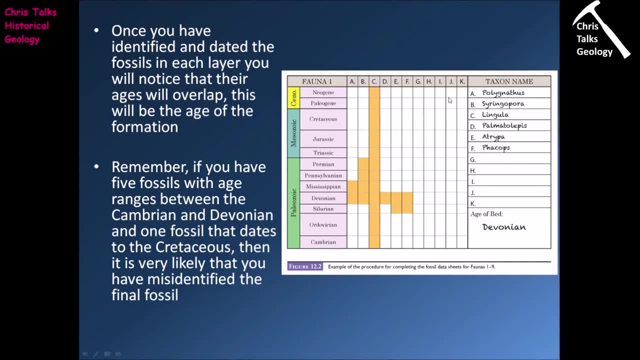 between here and here, and then you have one fossil that dates all the way up here, for instance in the paleogene. well, i think it's pretty fair to say you've misidentified that final fossil and you might need to go back into the textbook and maybe try again. so you know, just be smart. 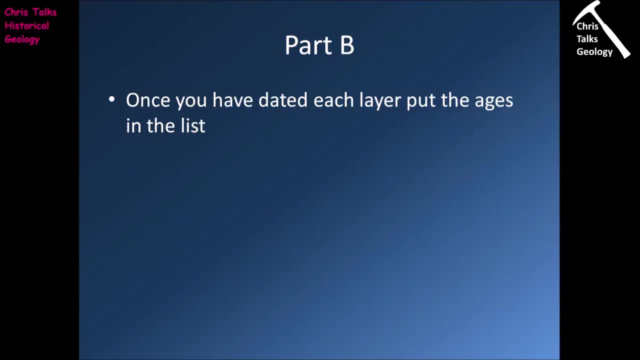 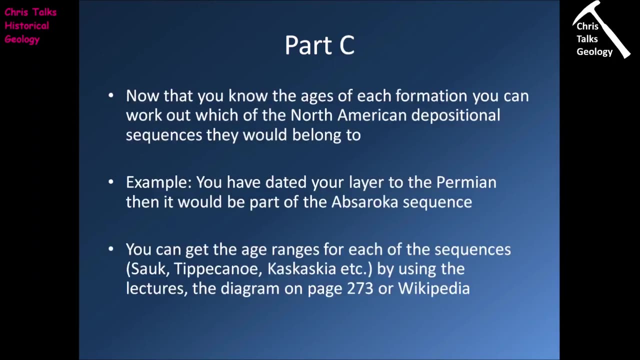 so once you've identified the fossils for each location and you've produced an age for each location, you're then going to write those ages into part b. so once you've dated each location, your next task is to try and work out to which north american depositional sequence your location belongs. 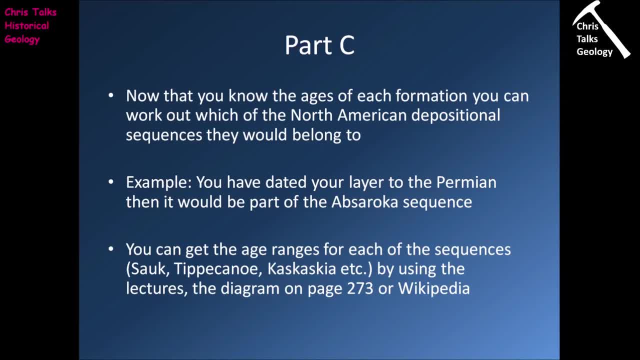 so the north american depositional sequences are, of course, the suk, the tipper canoe, the kaskaskia, the absaroka and the zuni. in this instance, we're not worried about the tehass. so how would we do that? well, obviously, let's say for one of the nine locations you've dated it to: 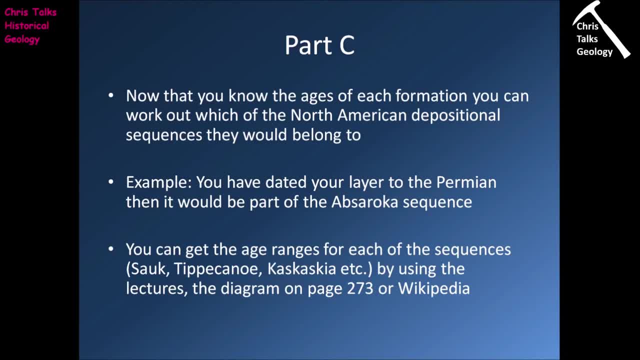 the permian. well, obviously the first depositional sequence that was forming in the permian was the absaroka, so therefore your location would be part of the absaroka sequence. so obviously you would then go to page 172, and on page 172 you can see part c, which is called depositional sequences, and then under number 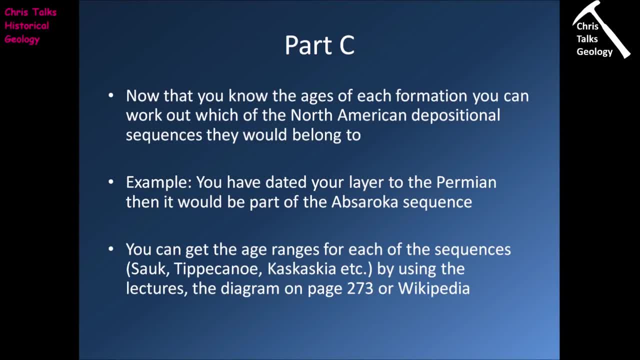 four, the absaroka sequence. you would write the name of your formation. it's all relatively straightforward, so you can get the age ranges for each of the sequences. so that's the suk, the tipper canoe, the kaskaskia, etc. the lecture material: the diagram on page 273 of ritter and peterson. 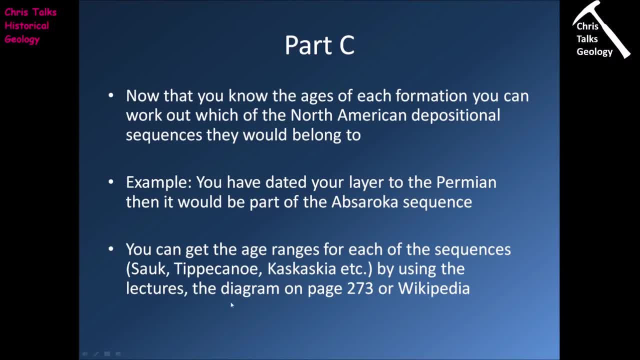 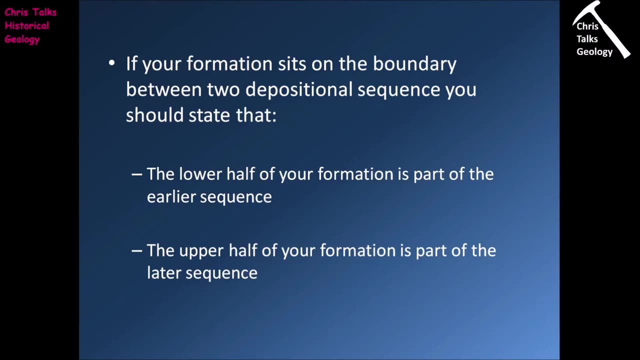 or wikipedia. so you know. just as long as you know the age ranges for each of the sequences, you can work out. you know which which sequence each location is part of. now, if it happens that your location is dated to an age that falls between two sequences, you're going to have to split your location up. so let's for argument. 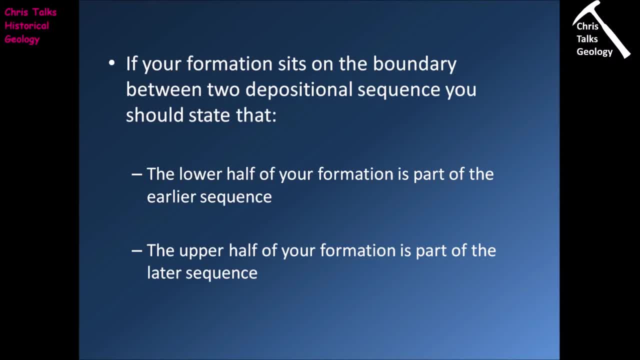 sake, say that your location is dated to the order vision. well, if it's, if it's dated to the order vision, that means that it sits essentially on the boundary between the suk and the tipper canoe, and so how are you going to deal with that? well, what you're going to say is: you're going to see. 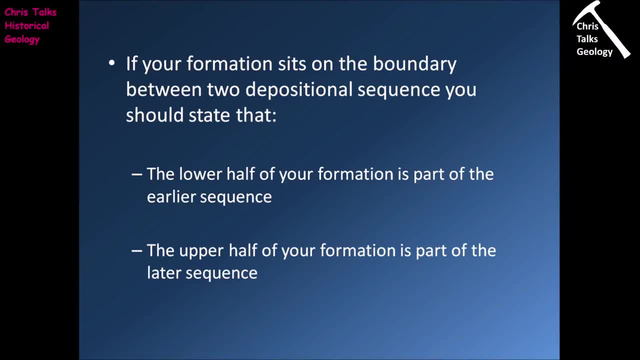 the say, the lower layers of your location are going to be part of the earlier sequence, that would be the suk. then the upper portion of your location is going to be part of the later sequence, that would be the tipper canoe, and so on. your diagram on page 100. on your diagram on on page 172: uh, under the soak sequence, you 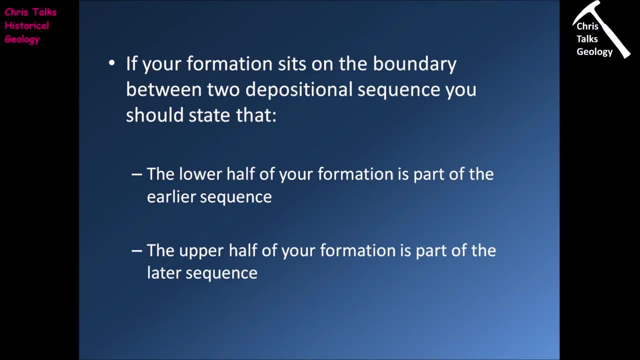 would write the lower portion of formation and then you would insert the name. and under the typical canoe, you would then write the upper portion of you know of formation and then you would insert the name again. so you would be simply stating that you know for each location. well, for, 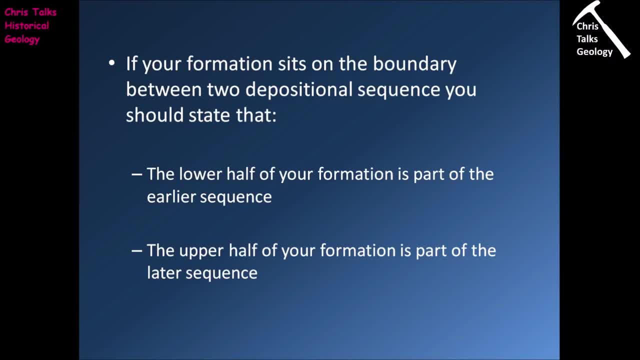 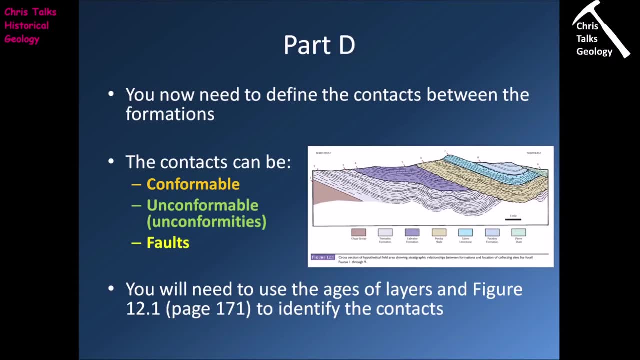 that particular location. half of it is part of the soak and half of it is part of the tipper canoe, and so on. you would have that final task, which is part d, which is to define the contact between the formations. so in the textbook it's going to ask you to define the contacts between several locations. 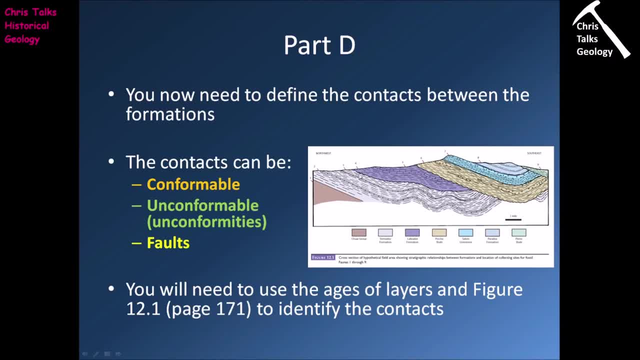 so let's say, for instance, between location 3 and location 4. it's going to be asking you what the contact, what's the nature of the contact, should i say, between these two formations? now, your contacts can either be conformable, unconformable, faults. So, in order to actually work out what the nature of the 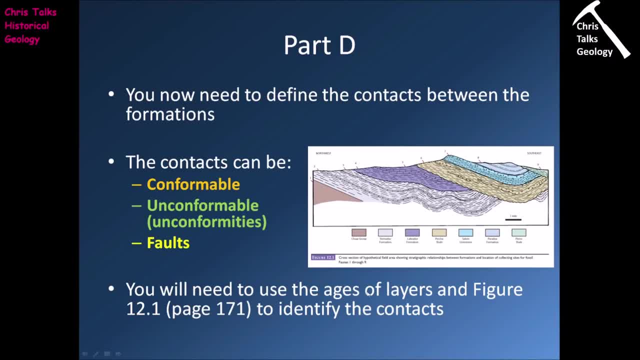 contacts are. you will need to use the ages which you've worked out for each of the locations and figure 12.1, which is this diagram right here. So use both of them to try and work out what you're looking at. So how are you going to? 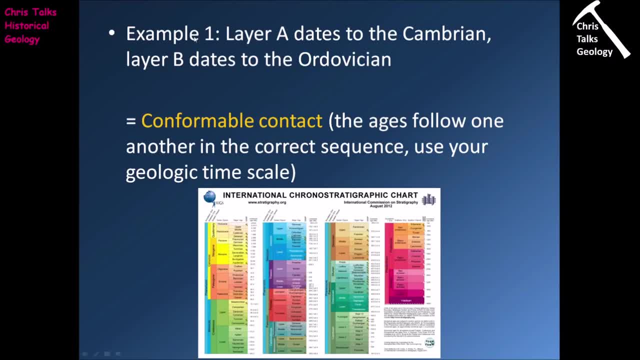 identify the nature of each contact. Okay, so example number one: layer A dates to the Cambrian and layer B dates to the Ordovician. Well, this contact is therefore going to be conformable because the ages are following one another in the correct sequence. so, in order to make sure you have the correct 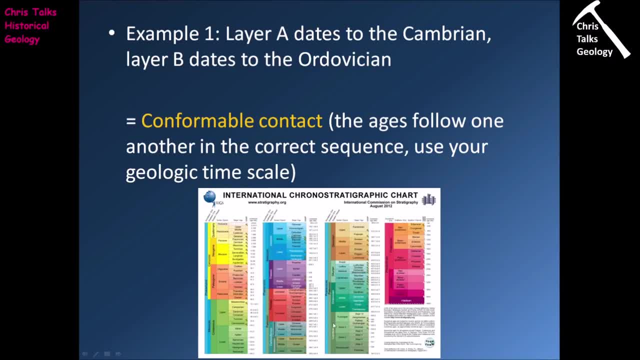 sequence. use your geologic time scale. So layer A would be down here in the Cambrian and layer B would be Ordovician, where we can see the Ordovician follows the Cambrian and therefore we can say that the contact between the two is going to be conformable. 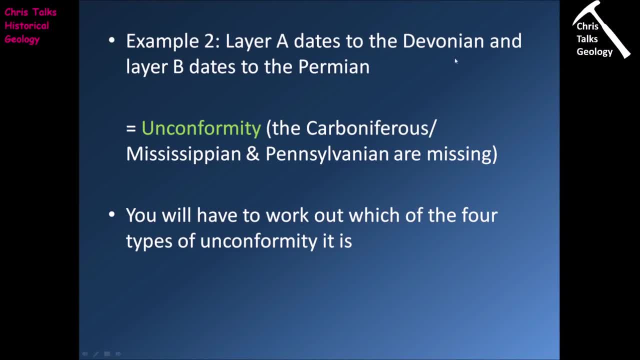 Now, in example number two, there are two different, two: layer a is going to date to the devonian and layer b is going to date to the permian. well, obviously, in that instance, we're missing some rock, aren't we? because we are missing the carboniferous. you know, it's not there, and so this means that the contact between layer a and layer 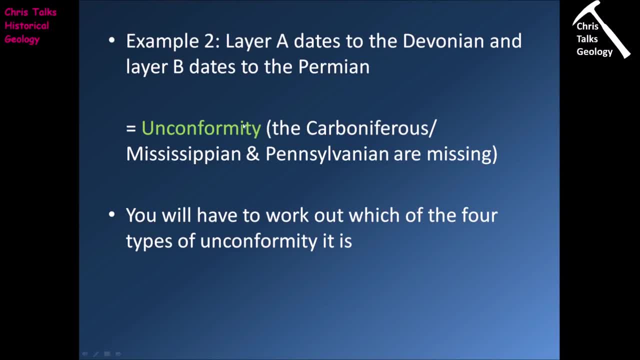 b must therefore be an unconformity. now, in terms of what type of unconformity it is, you're going to have to work that out for yourself. so, if you remember, there are four types of unconformity: disconformity, angular unconformity, non-conformity and paraconformity. so you're going to have to. 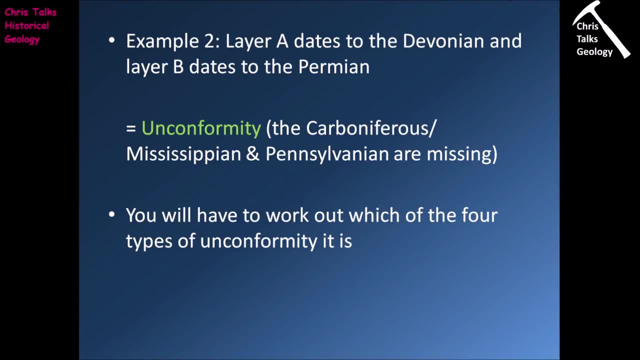 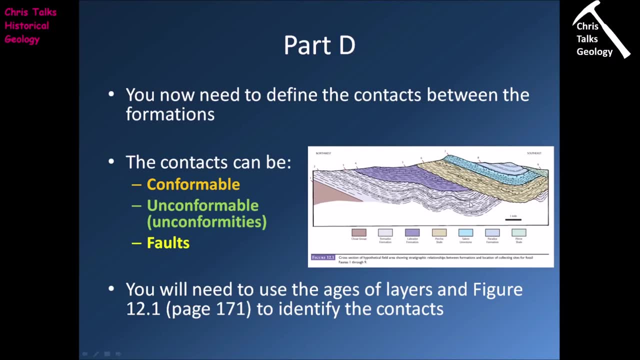 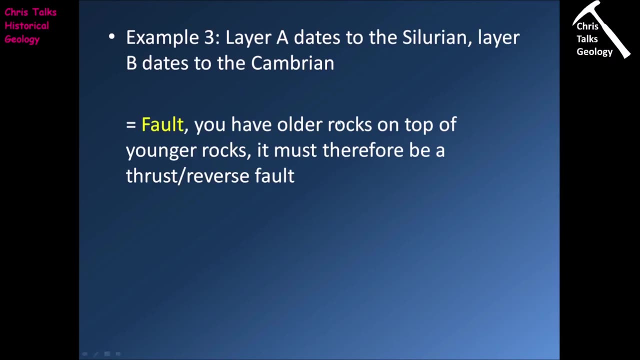 work out what type of unconformity you're looking at, and the way you're going to do that is by looking at figure 12.1. that's going to help you work out what type of unconformity it is. so the final type of contact you can have would be a fault. so in example three we're going to 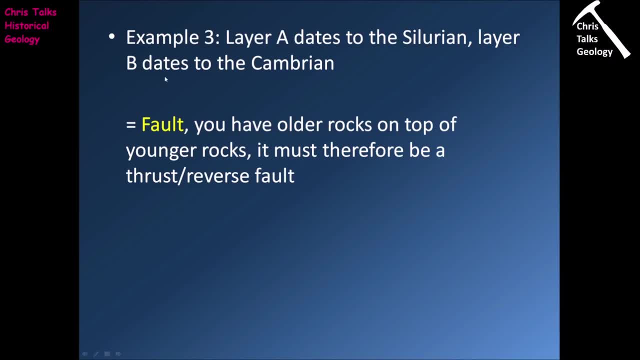 have layer a, dating to the silurian, and layer b, which is the decal promise. so we're going to have this analogous part of the area that we're going to be working around, then the superification and the decal from here. so you are going to have this squareango and then you're going to have this. 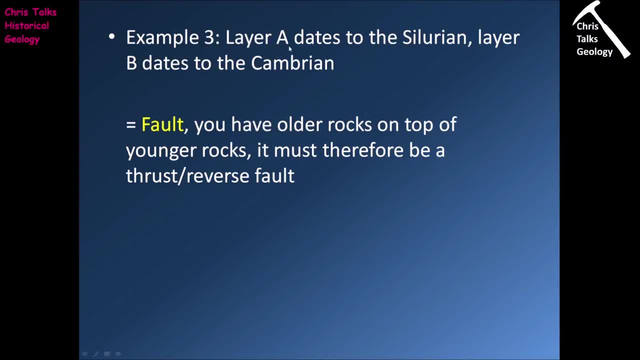 on top of it, dating to the cambrian. this means essentially, you have older rocks on top of younger rocks. now. this therefore means that the contact between the two must be a fault, and that fault will either be a thrust fault or a reverse fault, and that fault is therefore pushing older rocks. 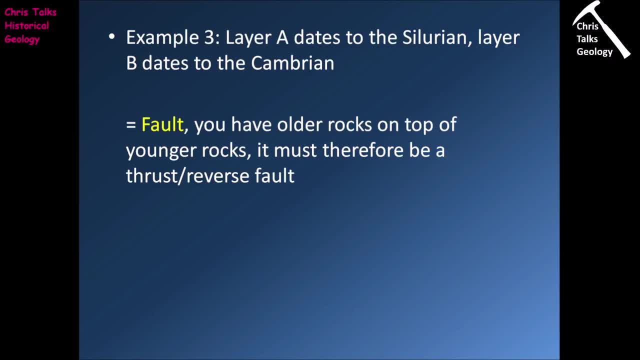 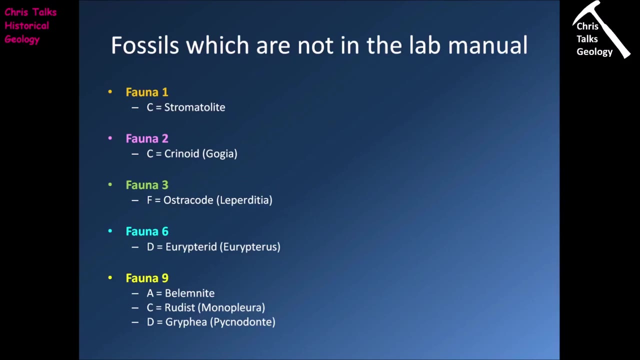 over the top of younger rocks, and so, for each of the, each of the different boundaries that are given to you as part of part d, your goal is to identify what the nature of each of those boundaries is. so the final slide here is simply a list of the fossils which are given to you. 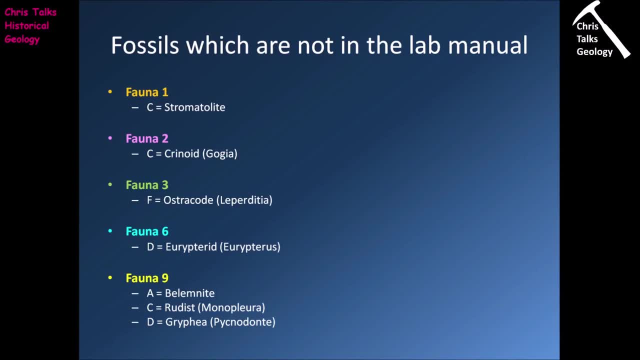 as part of the part a of the exercise, but they are not listed within the fossil data sheets. so you can see that for each of the locations of a fauna- 1, fauna 2, fauna 3, fauna 6 and fauna 9- i've listed the fossils which are not in the textbook so you can see for some. 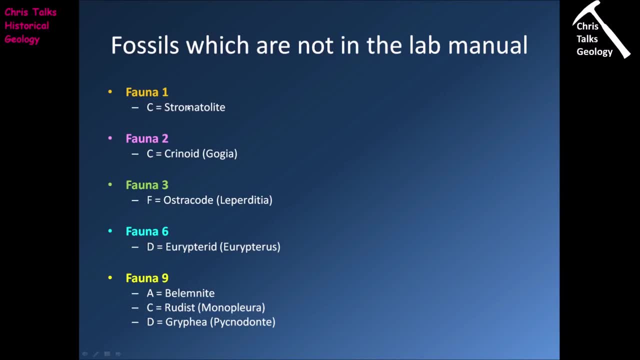 of them there's simply just a family name. so for instance here, stromatolite. but for some of them I've not only given you the family name, I've also given you the name of the individual species. so you'll find that in the brackets, and so if you're searching for the age range for this particular,